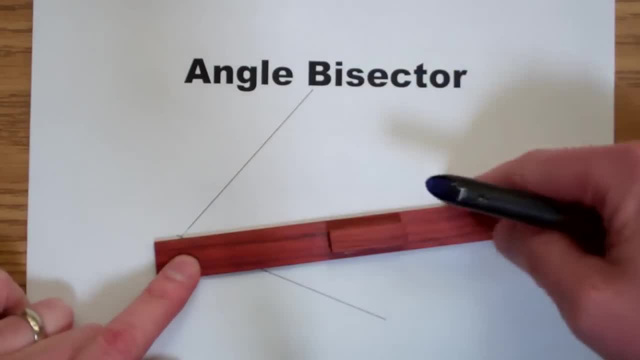 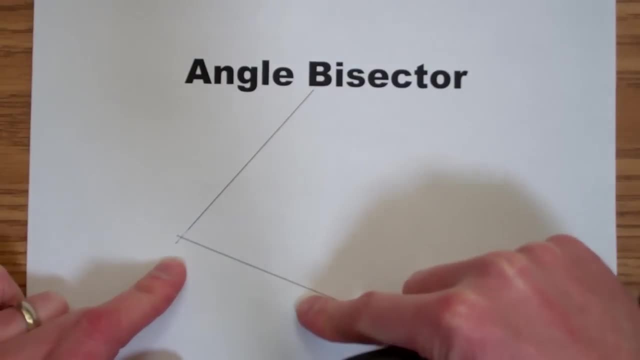 is going to go somewhere through the middle. here, All the points on the angle bisector are equidistant from each side of the angle, So we know that it's going to go through the vertex and we need one more point to determine this line. 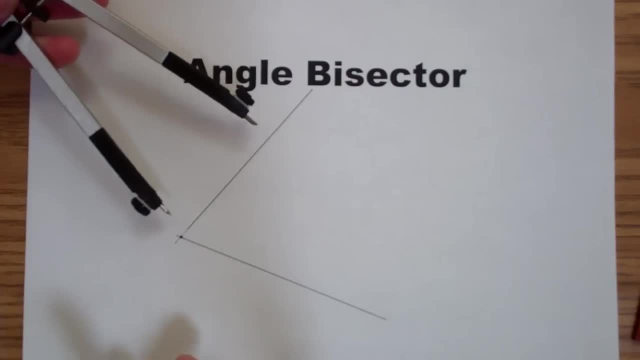 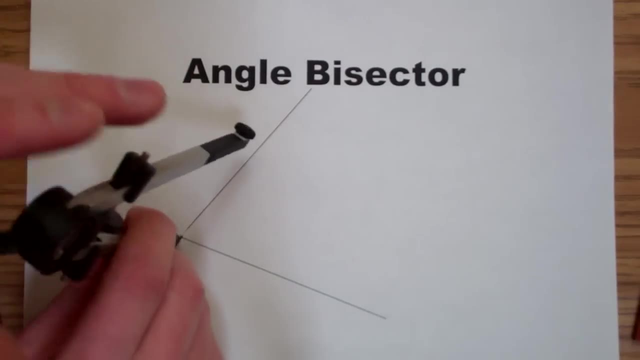 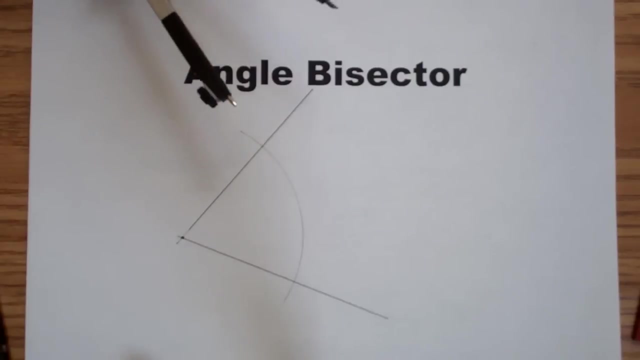 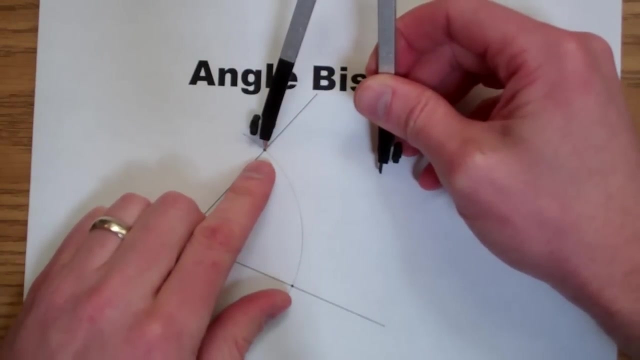 To find this point, we'll start by setting our compass so that it will intersect both sides of the angle and then drawing that arc. Now we've created two new intersections, here and here, And from those intersections we're going to take our pointer and stab in. 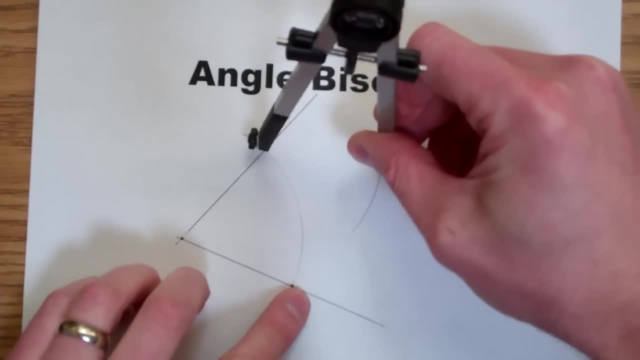 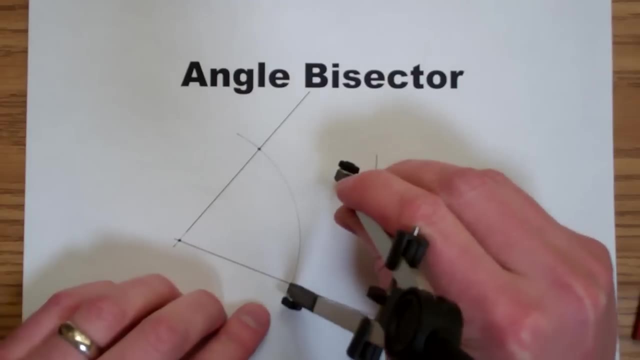 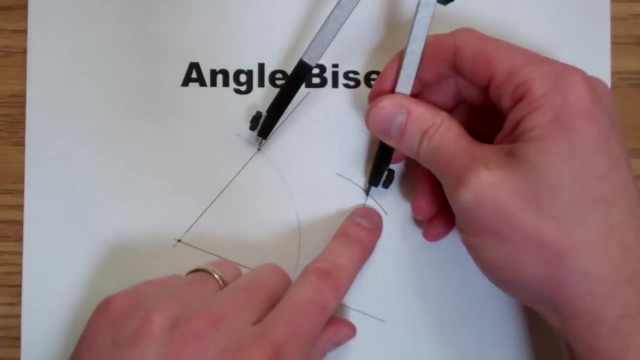 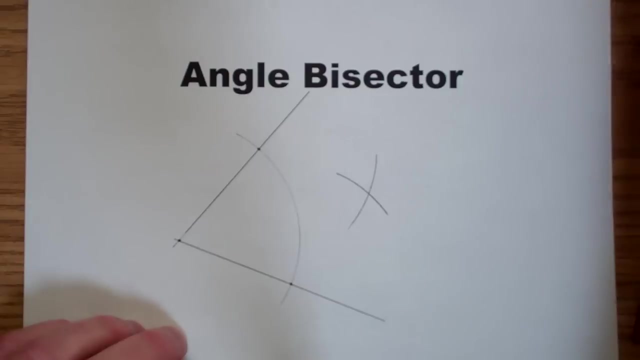 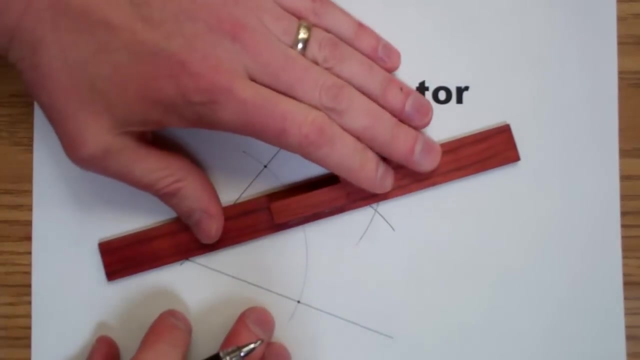 and draw arcs in the middle of the angle, One here and one from the other side, So that those arcs intersect. Now this new point is equidistant from both this side and this side of the angle. To complete this construction, we use our straightedge to connect the vertex. 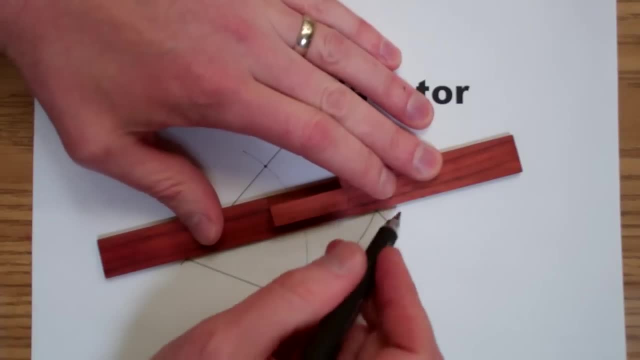 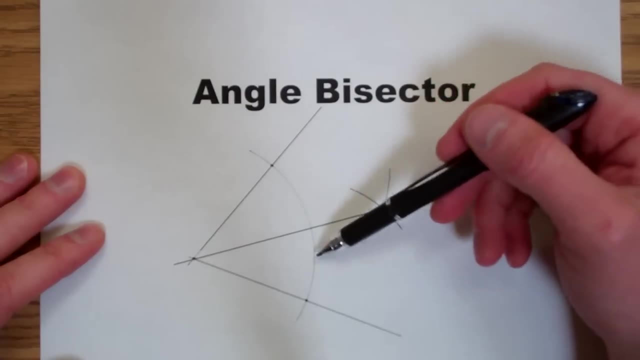 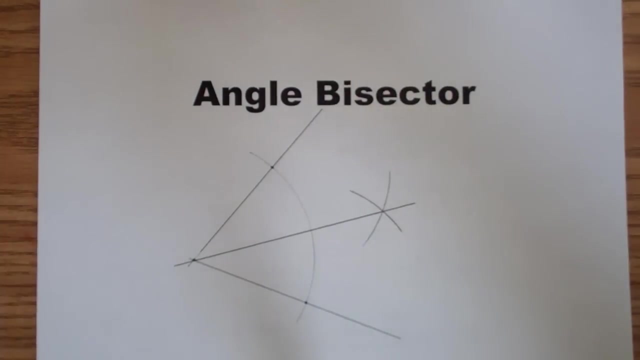 and this new point. Now we have two congruent angles bisected by this line. 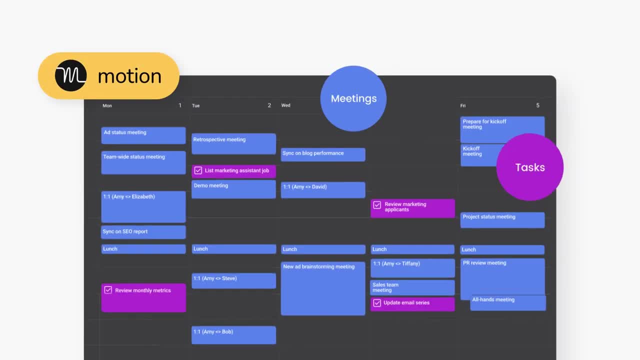 What's the difference between Motion and Reclaimai? Motion is designed strictly for making time for your tasks. It wasn't built to help teams manage their work. Reclaim gives you powerful controls for your one-on-one meetings, automatically scheduling across two busy calendars. 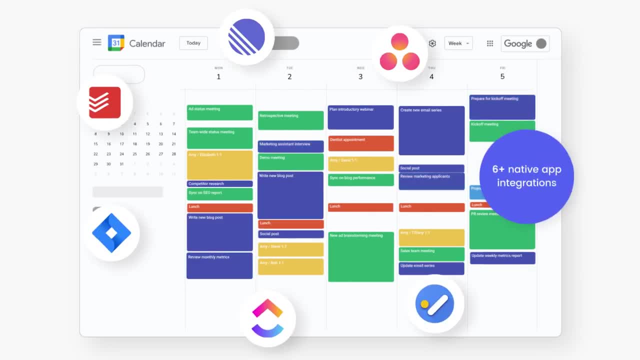 and integrates with more of the tools your teams use, like Jira, Asana, Linear, Todoist, ClickUp and Google Tasks, where Motion forces you to recreate your task list from scratch. Reclaim also gives you more ways to try before you buy. 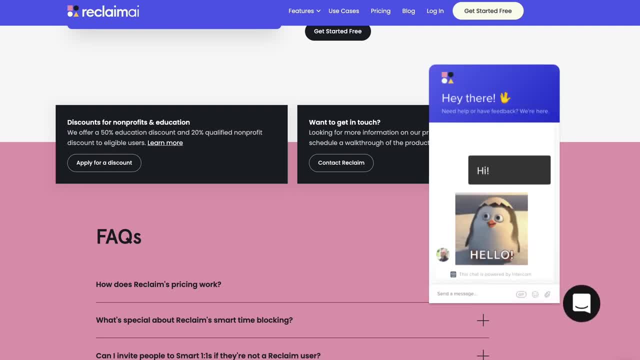 with a robust free plan, flexible pricing options and real-time customer support for teams of all sizes. Motion only gives you a seven-day trial, offers no free plan and costs nearly four times as much per month. Many more advantages to check out at Reclaimai. 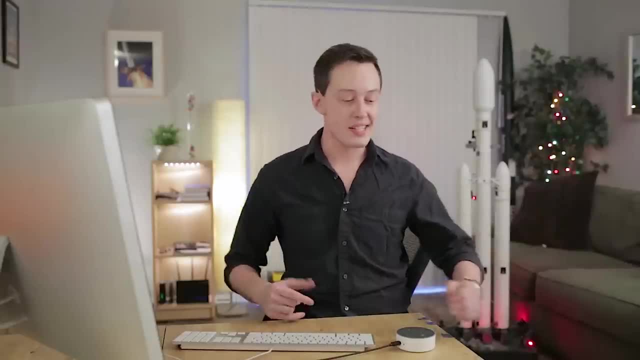 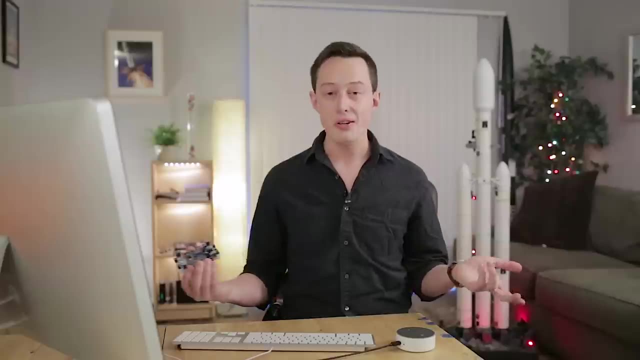 Hi everyone, my name is Joe Barnard. Welcome back to Landing Model Rockets. This is episode 8, where we're going to start working on the code and flight software for the blip computer. There are going to be several episodes about code and this is just the first in those.